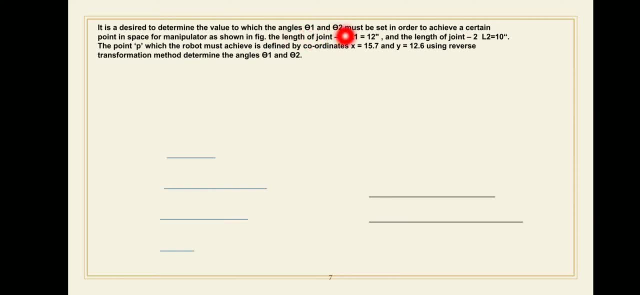 value to which the angle theta 1 and theta 2 must be set in order to achieve a certain point in space for manipulator. as shown in figure, the length of joint 1 means L1 is given. L1 is 12 inch and the length of joint 2, L2, is 10. then the point P which the robot must achieve is defined by: 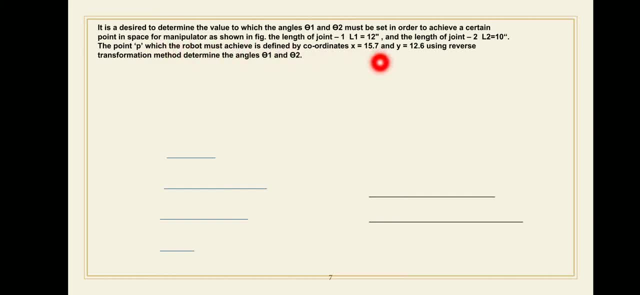 coordinates means Cartesian space coordinates are defined by coordinates of L1 and L2.. given X is equal to 15.7 and Y is equal to 12.6, using a reverse transformation or inverse transformation method, determine the angle. theta 1 and theta 2 means you have to find out the angle. 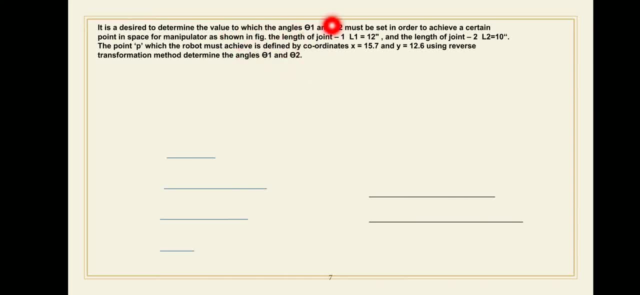 theta 1 and theta 2, and these are the different given parameters. for given parameters means length of joint 1, L1. length of joint 2, L2, then X or Cartesian space coordinates X and Y. so in this figure two joints are given or two lengths are given, two links, link number. 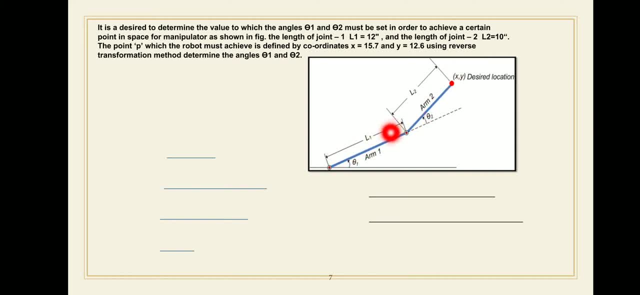 first link number. second, L1 is the length of link number first and L2 is the length of link number second. theta 1 is the angle between axis of link number first and horizontal distance. theta 2 is the length of link number second. and P X comma Y is the desired location. so this is the known point. 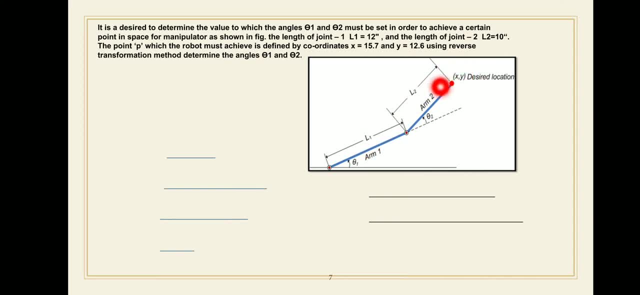 or given point. so L1, L2 and X and Y coordinate. these are the given parameters and you have to find out angle: theta 1 and theta 2 respectively, okay, or transformation method: determine the angle: theta 1 and theta 2.. so first of all, you have to write the given data. 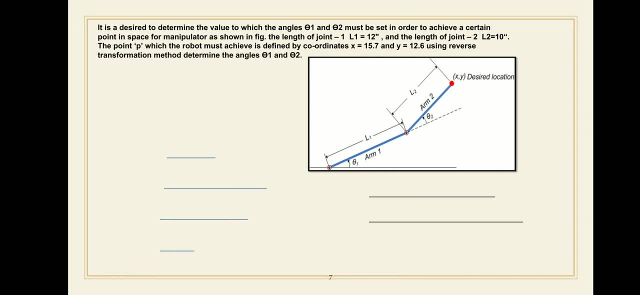 or all given parameters in problem statement. so, given values L1 is 12 inch, then L2 is the 10 inch, then X and Y coordinates given. means Cartesian space coordinates are given: X is equal to 15.7 and Y is equal to 12.7. means these are the given parameters or Cartesian space parameters are given. 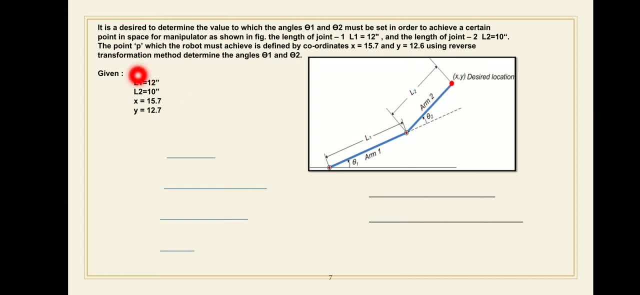 and links are given. so four given parameters and you have to find out the angle. theta 1 means angle made by axis of link number first and horizontal, and theta 2 is the angle between axis of link number first and link number second. so these are the two findings of inverse kinematics problem: theta 1 and theta 2. 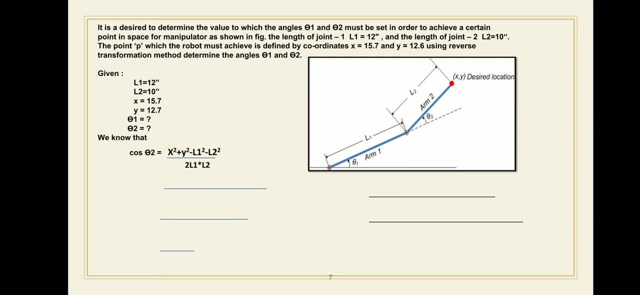 so we know that the formula for theta 2, or how you can find out angle theta 2, we already discussed in previous lecture. or how you can find out the angular position or angular space parameters by using inverse kinematics. so this is simply equation. by using this equation, you can easily find out angle theta 2. angle theta 2 is equal to cos. 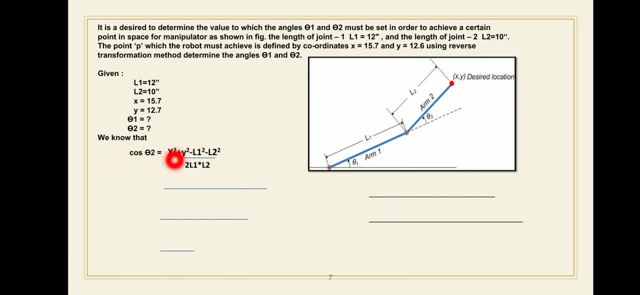 inverse of answer means: cos theta 2 is equal to X square plus Y square minus. here L1 square minus L2, square upon 2 into L1, into L2. this is the simply equation. by using this equation you can easily find out angle theta 2. so put all given values, this four given values, and find out. 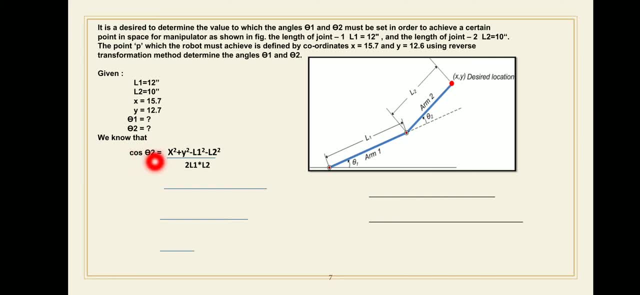 angle theta 2, so cos theta 2 is equal to X square, X square is the 15.7, Y square is the 12.7 minus L1 square is 12.7.. and L1- L2 square is the 10 divided by 2, into L1. L1 is 12 and L2 is L2 is 10. so put all given values 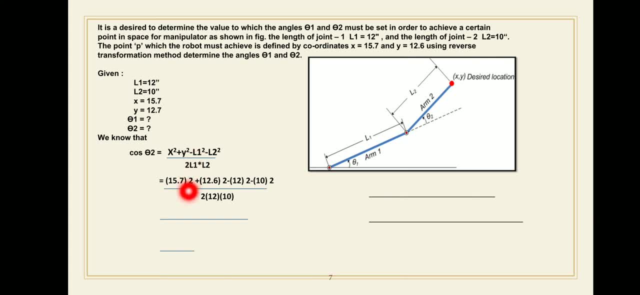 15.7 into 2, or 15.7 square plus 12.7 square minus 12, 12 square minus 10 square upon 2 into 12 into 10. so solve this equation and finally we get this answer to 46.5, 158.76 minus 144 minus 100 upon 2 into 12 into 10.. 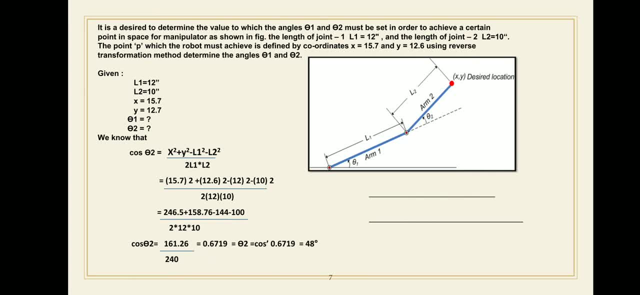 so this is the final answer. cos theta 2 is equal to 161.26 upon 240. means cos theta 2 is equal to 0.6719 or theta 2 is equal to cos- inverse of answer, of course, inverse of 0.679. so after solving this equation, we can directly get the angle: Theta 2 or. 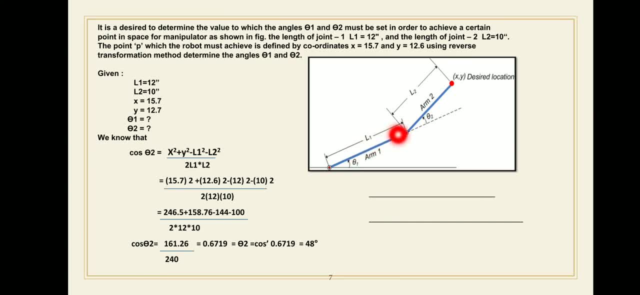 angle. Theta two means uh, angle between axis of link number first and link number second. Theta 2 is equal to 48 degree. this is the first finding or first answer of inverse kinematics of two degrees of freedom robot. then what is your next answer of inverse kinematics of two degrees of freedom robot? then what is your next? 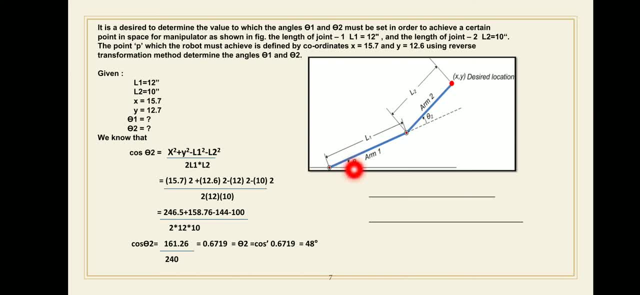 objective. you have to find out angle theta 1 means angle made by axis of link number first and horizontal plane. so we know that formula for inverse kinematics or to find out angle theta 1. so this is the simple formula to find out angle theta 1. time theta 1 is. 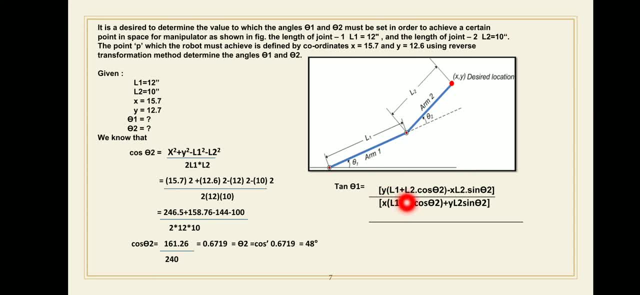 equal to y into l1 plus l2, cos theta 2 minus x into l2, sin theta 2. okay, divided by x into l1 plus l2, cos theta 2 plus y into l2, sin theta 2, put all given values, means this four: 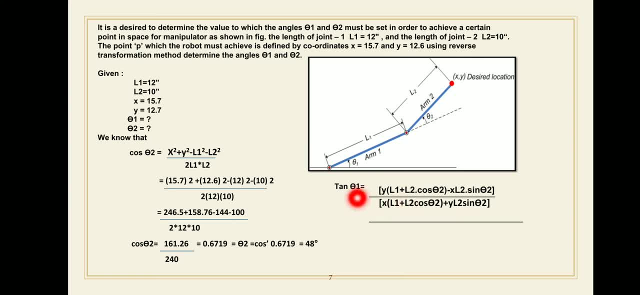 given values in this equation and find out angle. theta 1 means theta 1 is equal to tan inverse of answer. tan inverse of answer is equal to tan inverse of answer of this, all quantities or all parameters. so put this: all given parameters, y is 15.7. 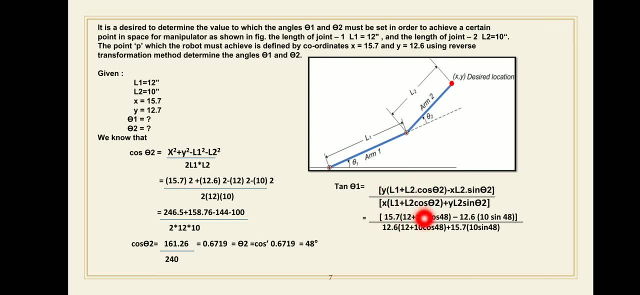 then l1 is nothing but 12. l2 is 10 cos. theta 2: theta 2- this is the answer for theta 2- 48 cos 48 minus x into l2, 12.6. l2, 10 sin 48, theta 2 is 48.